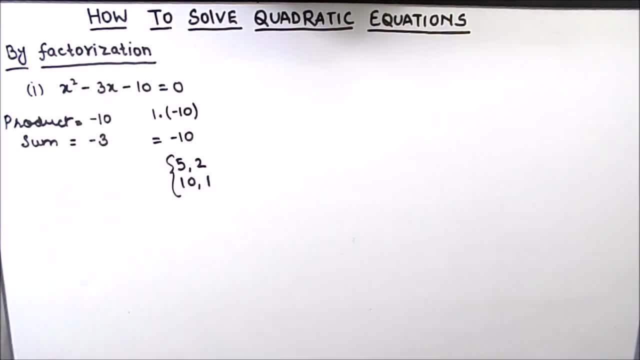 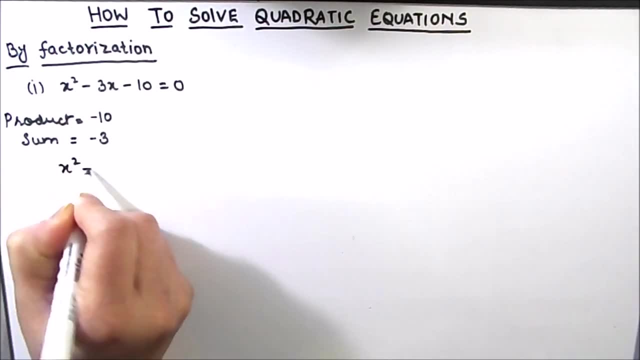 3, the coefficient of x or the middle term. The factors which satisfy these conditions are 5 and 2.. So now we will take our equation, we are going to break this middle term and write it in terms of 5 and 2, which are the factors of negative 10.. So here, minus 5x and minus 2x will give us minus. 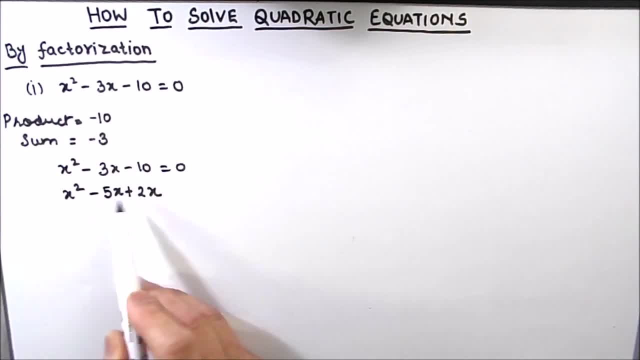 3x and their product negative. 5 and 2 will give us negative 10.. So both the conditions are satisfied. now we can write negative 10 and can solve it further. So out of these two terms we are going to take x common. so this will be x, x minus 5. and out of these two terms we can take 2 common. 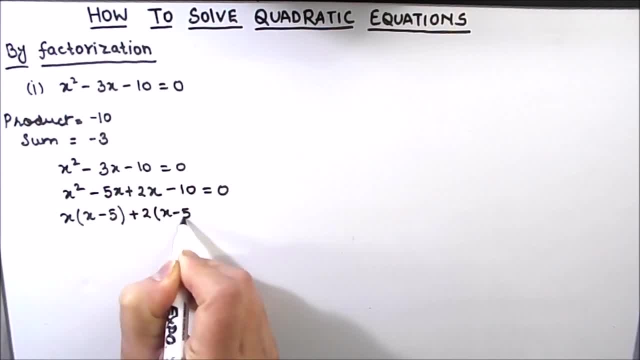 so plus 2 x minus 5 is equal to 0.. Now one more thing is that you can write 5x and 2x in any sequence. you can write plus 2x minus 5x or minus 5x plus 2x. 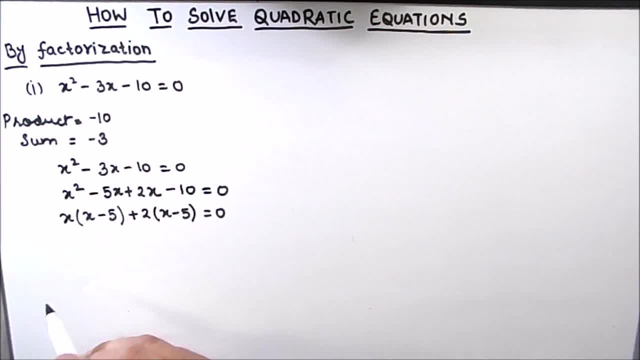 That will not going to change the solution or answer of the equation. Take x minus 5 as common, so x minus 5, and here we are going to left with x plus 2.. For finding the roots, either x minus 5 is equal to 0. from this we will get x is equal to 5. 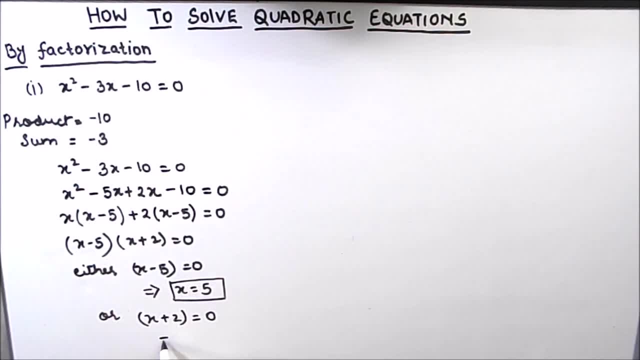 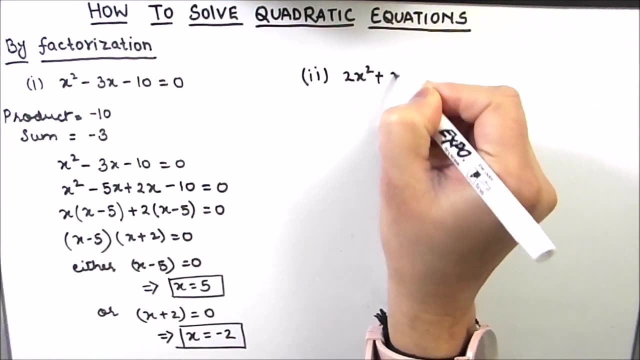 2 is equal to 0.. From this we are going to get: x is equal to negative 2.. Two roots of the equation are negative: 2 and 5.. Our second example is 2x square plus x minus 6 is equal to 0. So the 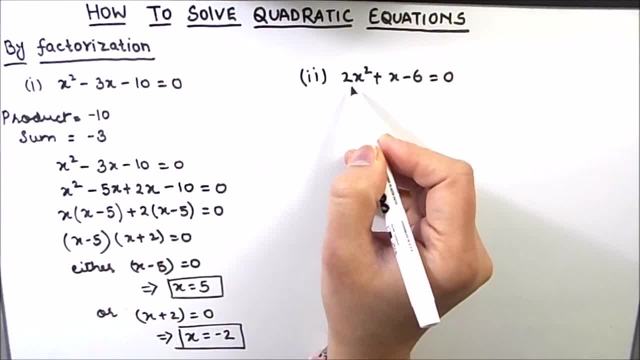 difference between this equation and this equation is that in the second equation we have coefficient of x square as 2, whereas in the first equation we have coefficient of x square as 2.. So in the second equation we have coefficient of x square as 1.. First we are going to take the product of. 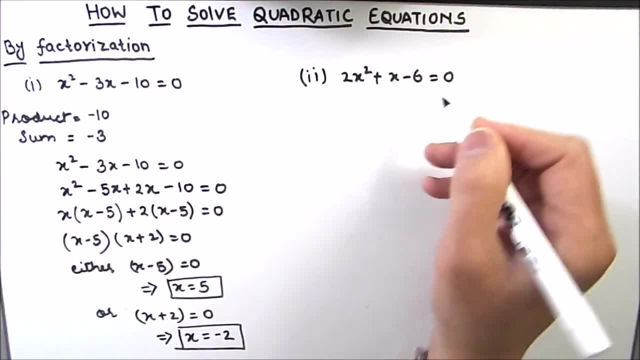 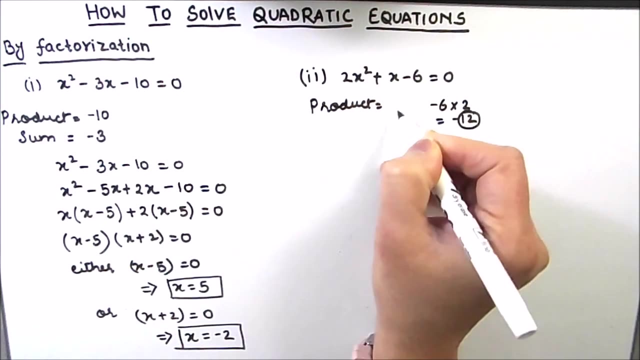 coefficient of x square and the last term, which is the constant. So the product is negative 6 times 2, which is equal to negative 12.. Now we need to find the factors of 12, such that their product is equal to negative 12 and their sum is equal to. 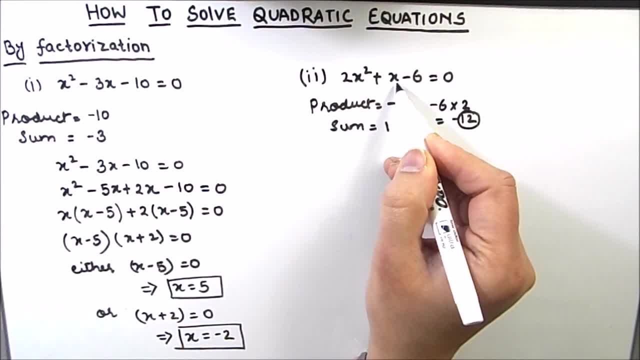 1, which is the coefficient of x square. So we are going to take the product of x square and the last term, which is the coefficient of this middle term, x. The factors of 12 are 6 and 2,, 3 and 4,, 12 and 1.. So, out of 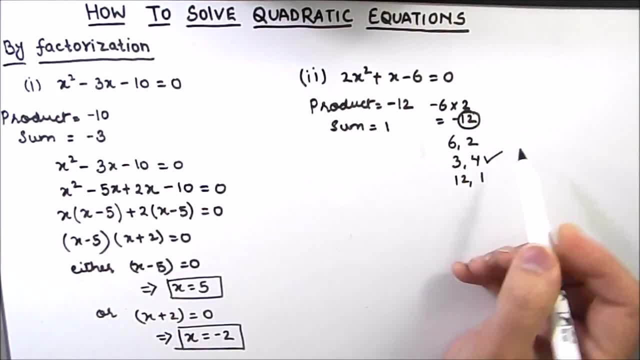 these factors, the only factors which satisfy the condition of product as negative 12 and sum as 1, are 3 and 4.. So we are going to take 3 and 4 as the factors We need, plus 1. so we are going to take. 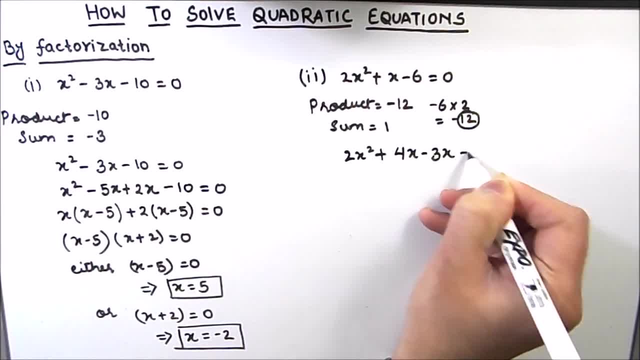 plus 4x negative, 3x negative 6 is equal to 0. minus 3x is equal to x, and 4 times negative 3 is equal to negative 12. both the conditions are satisfied. now we can solve it further, so we can take 2x common here. so this will be x plus 2. 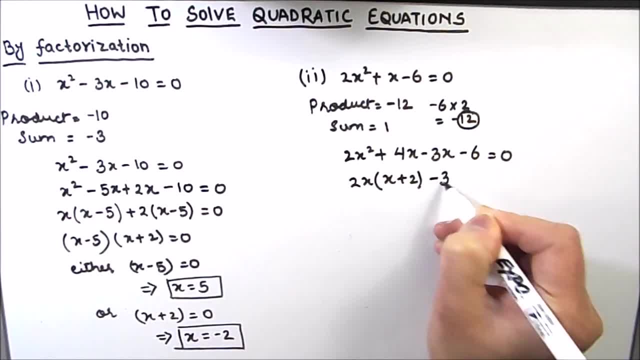 and from here we can take minus 3 common, so this will be x plus 2. so out of these two we can take x plus 2 common and the other term will be: 2x minus 3 is equal to 0, now either x plus 2 is. 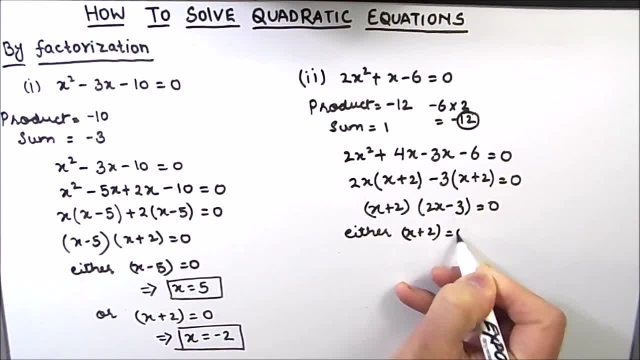 equal to 0, which will give us x as equal to negative 2, or 2x minus 3 is equal to 0, from which we will get x is equal to 3x divided by 2, or 3 by 2.. So these are the two roots of this equation. So here we have solved. 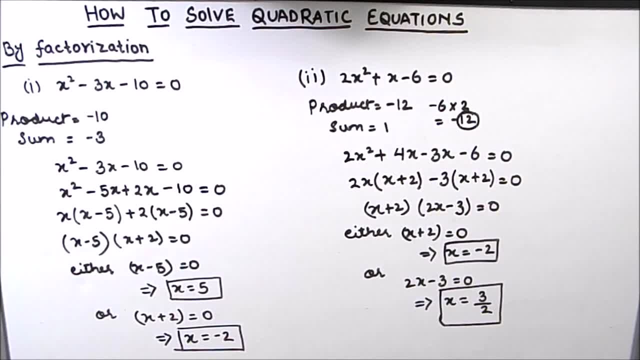 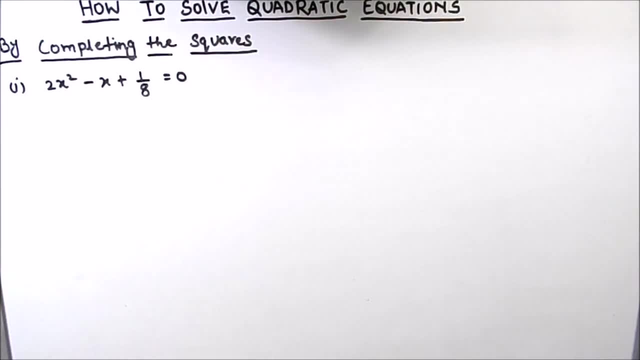 the quadratic equation using the method of factorization. Let's move on to our second method of solving quadratic equation, which is by completing the squares. So our first example in solving the quadratic equation by completing the squares is 2x square minus x plus 1 by 8.. 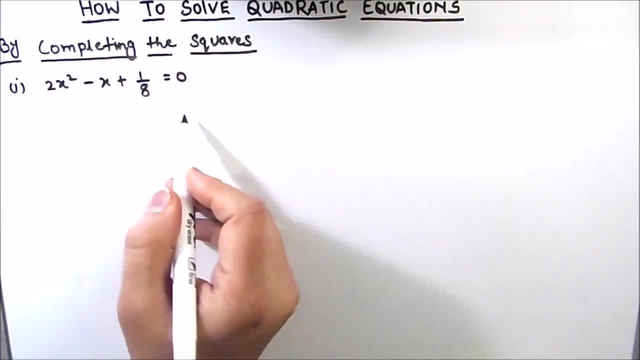 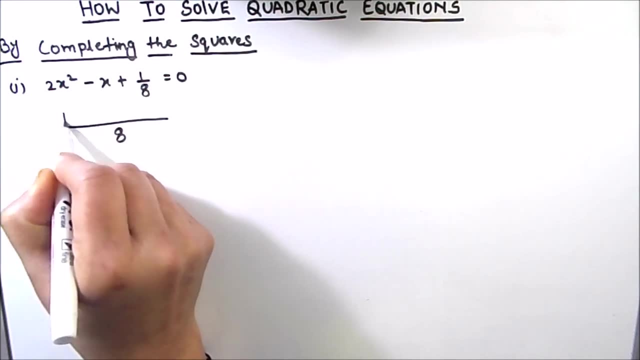 As there is a fraction in the equation, we can take the LCM and can simplify this. So LCM will be 8.. So this will become 16x square 8 times 2 is 16 minus 8x plus 1 is equal to 0.. Now we will. 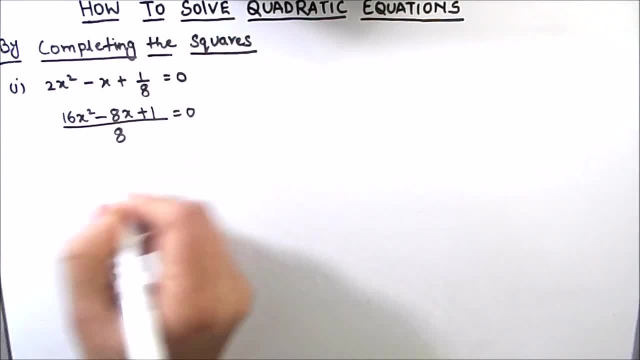 cross multiply, So this 8 will get multiplied to 0 and we are left with 16x square minus 8x plus 1 is equal to 0. This is our quadratic equation and we need to find the solution of this equation by completing. 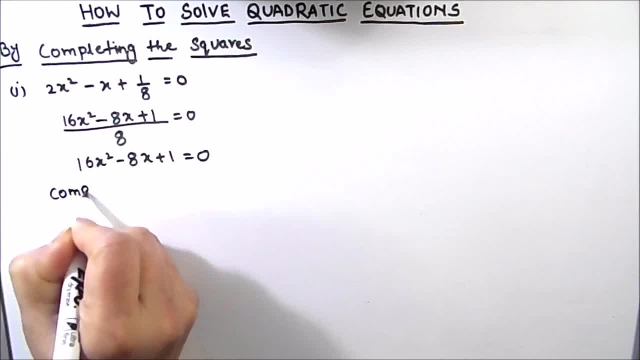 the squares. Now we are going to compare this equation with the whole square equation, which is a plus b whole square is equal to plus 2ab plus b square. Now we have a square term as 16x square, So we can write it as 4 times x. 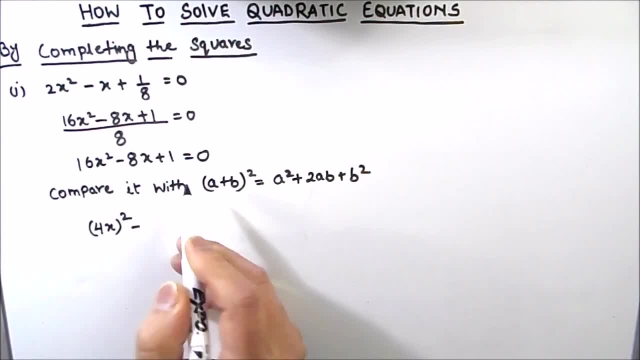 whole square minus this is 8x and we need to write it in terms of 2 times a times b, So we can write it as 2 times 4x, x. a is 4x and b as it is 8x and our term is complete, so b should be 1. 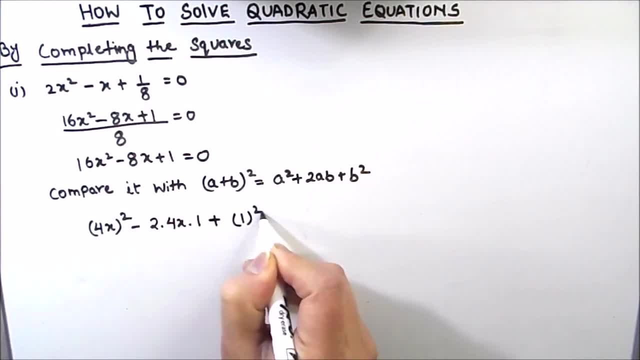 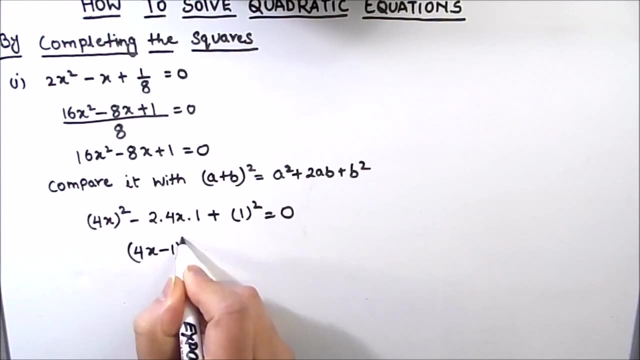 plus 1 square is equal to 0. So this is of the form a square plus 2ab plus b square, So it can be written as a plus b whole square. as it is negative 2, so this will be: 4x minus 1 whole square is equal to 0, which is equal to 4 x minus 1 times 4 x minus 1 is. 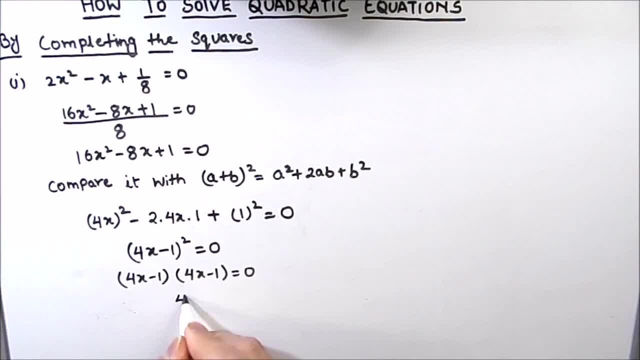 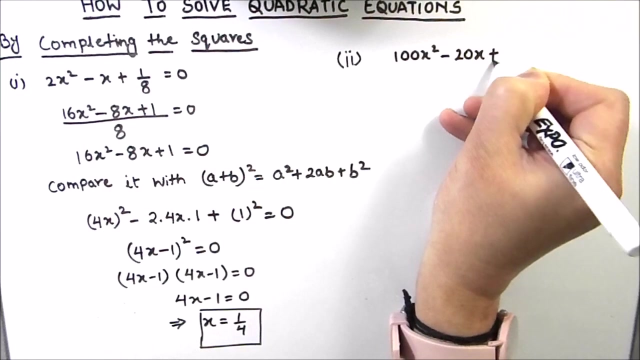 equal to 0. Both the roots are equal, so equation will have only one solution: 4 x minus 1 is equal to 0, which will give us x is equal to 1 by 4.. Let us solve one more example to clarify this further. So our second example is 100x square minus 20x plus 1. 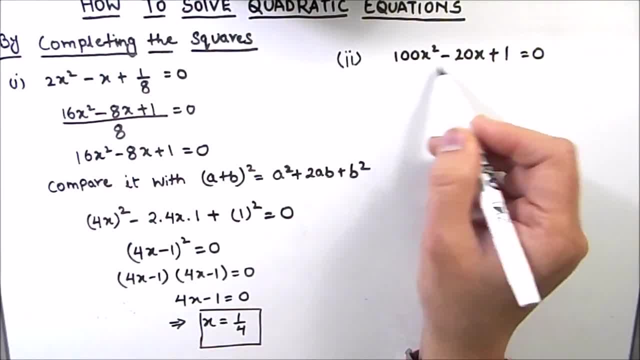 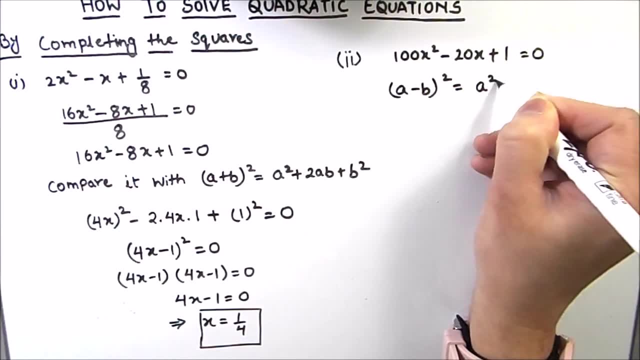 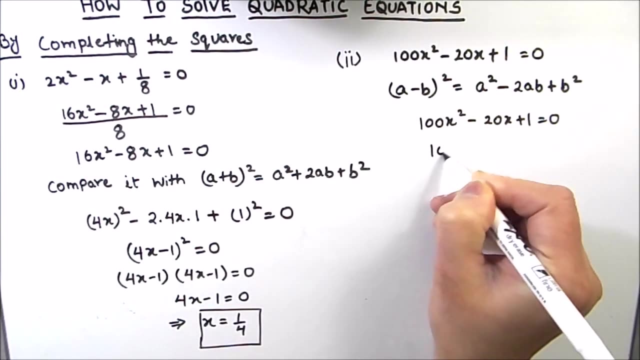 is equal to 0.. So here too we are going to compare this equation with a minus b whole square. So a minus b whole square is equal to a square minus 2ab plus b square. So first term is 100x square, which can be written as 10x whole square. The middle term is 2 times a times b, So we can write: 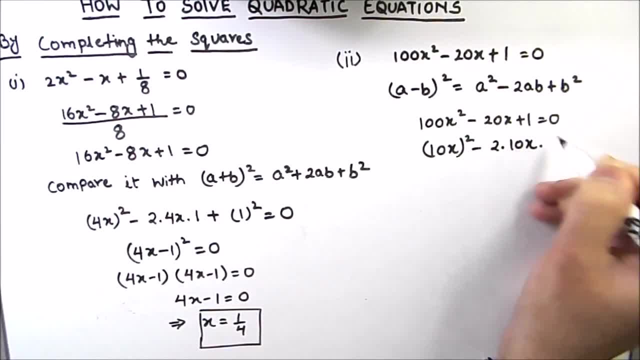 it as 2 times 10x times b will be 1, because 2 times 10x is 20x and we got the middle term. So our third term, or the b square term, will be 1 plus 1. whole square is equal to 0. So this is of. 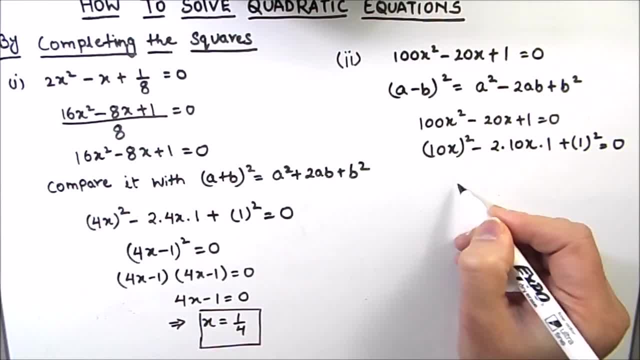 the form a square minus 2ab plus b square, which can be written as a minus b Whole square, or 10x minus 1 whole square, which is equal to 10x minus 1 times 10x minus 1 is equal to 0.. So this also will have only one solution to the equation, which is same and 10x minus 1. 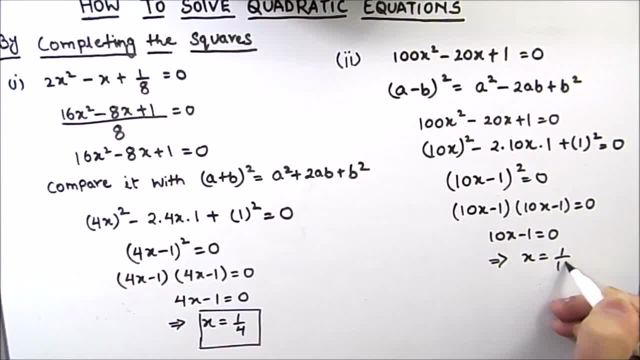 is equal to 0 will give us x is equal to 1 by 10.. So this is the solution to the equation. This is the second way In which we can find the solution to the quadratic equation. Now we will solve few examples of the last method of solving quadratic equation, which is by using the quadratic formula. 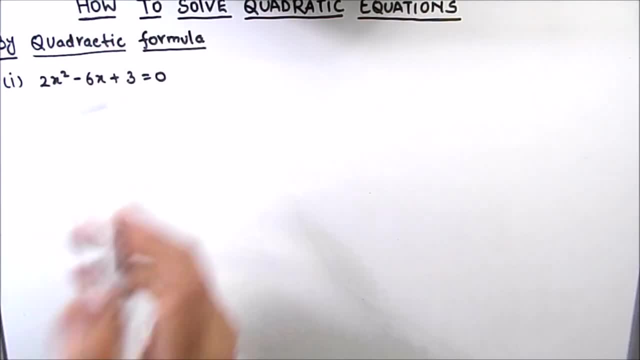 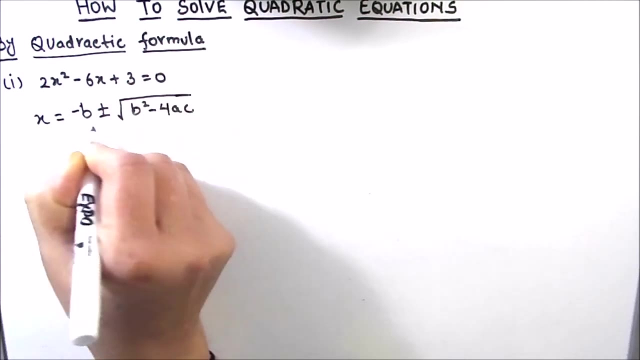 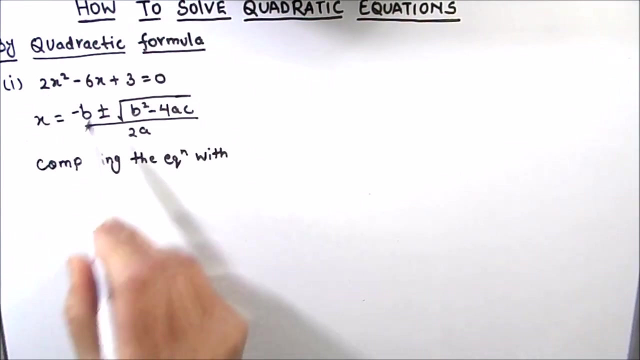 So our first equation is 2x square minus 6x plus 3, and the quadratic formula we are going to use is: x is equal to negative b plus minus under root of b square minus 4ac divided by 2a. So first we will find a, b and c in the equation. So we are going to compare this equation with: 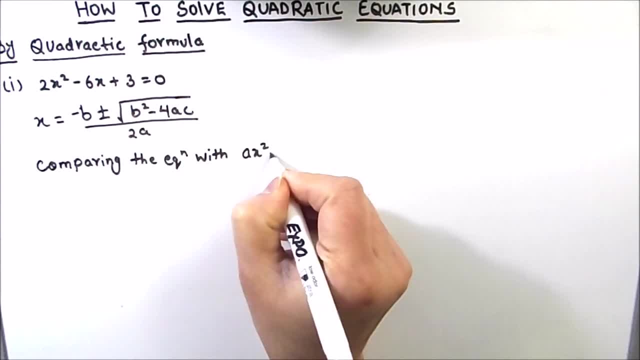 standard quadratic equation, which is ax square plus bx plus c, is equal to 0.. So by comparing we are going to get a as 2, b is equal to negative, 6 and c is equal to 3.. Now we will substitute these values in the formula, So x will be equal to minus b. 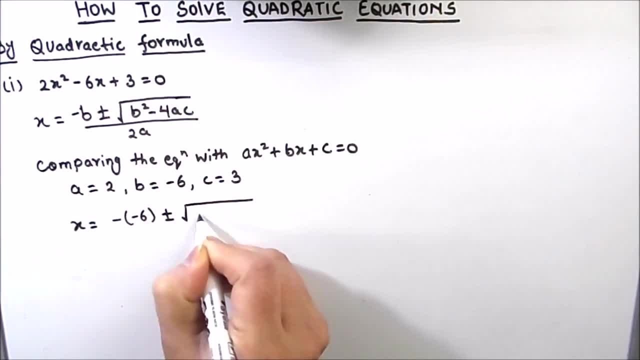 Plus minus b, square minus 4 times a times c, divided by 2 times a, which is 2, so negative times negative, 6 will be 6 plus minus. square root of 36 minus 4 times 2 is 8, 8 times 3. 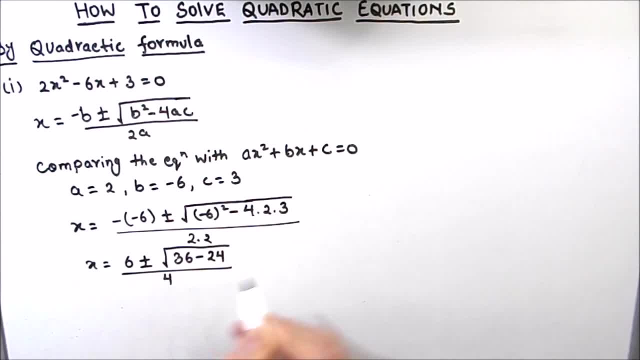 is 24 divided by 4.. so this will be equal to six plus minus 36. minus 4 times 3 is 24.. So 4 times 6 is equal to 3, as 3 is 4.. I will leave theseобщ, which are going to be none but thousand eye verse. 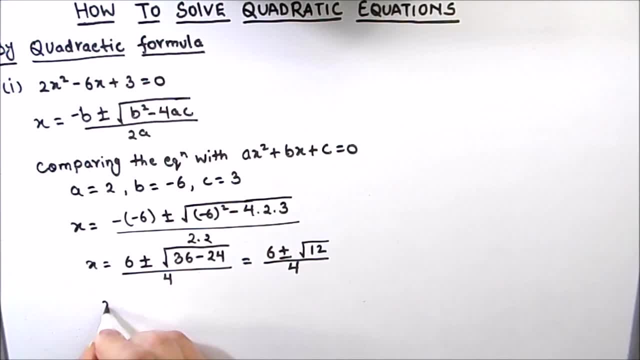 minus 24 is equal to 12, so x is equal to 6 plus minus 12. can be simplified as 3 times 4 divided by 4, and this 4 will come out. so this will be 6 plus minus 2 root 3 divided by 4. we. 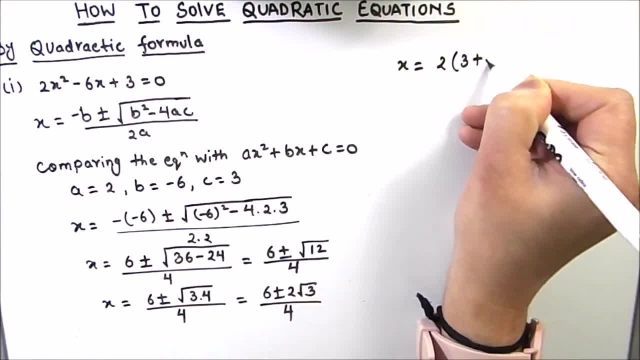 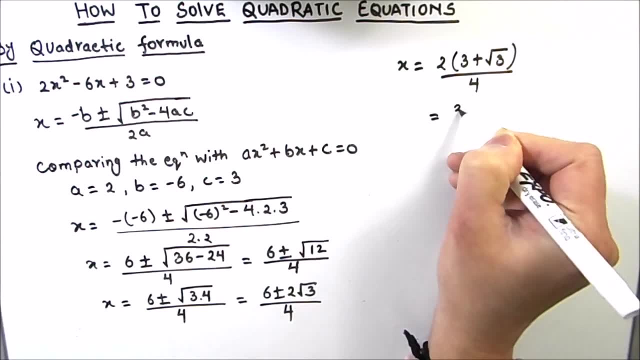 are going to take 2 common here, so this will be 3 plus root 3 divided by 4, and this 2 and 4 get simplified to 3 plus minus- sorry, plus minus root 3 divided by 2. so now we have either: 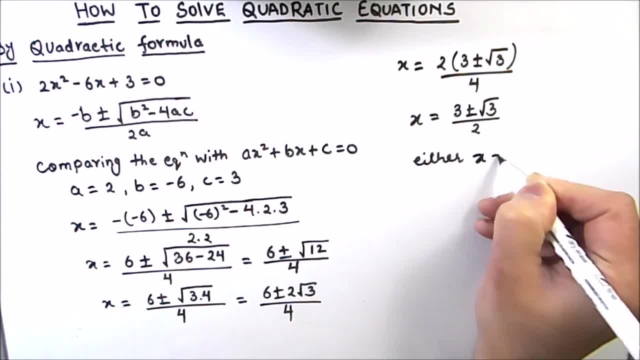 x is equal to 3 plus root 3 divided by 2, or x is equal to 3 minus root 3 divided by 2. these are the two solutions to this equation. this is how we can use quadratic formula and find the solution. let us solve one more example and 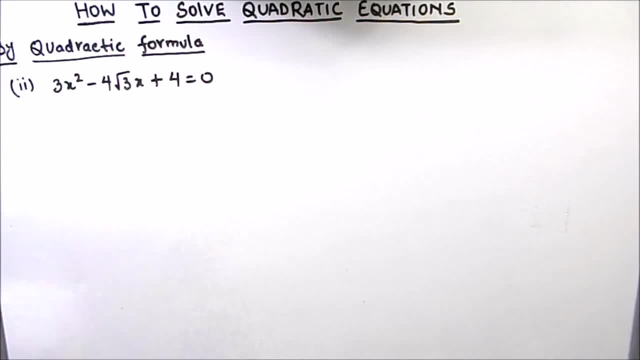 find the solution to the quadratic equation. so our first step is to compare this equation with the standard equation. the standard equation, which is ax square plus bx plus c, is equal to 0, 0.. So we are going to get a as 3, b as negative, 4 root 3 and c as 4.. Now our formula is: x is equal.